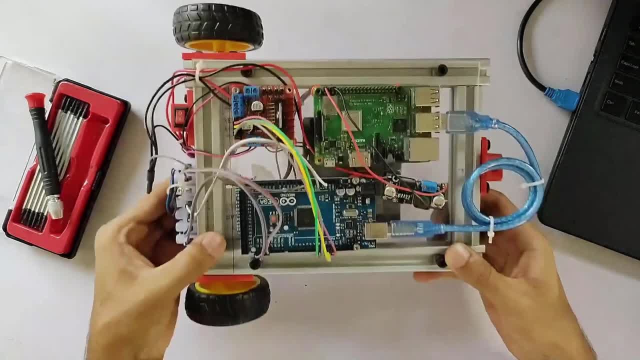 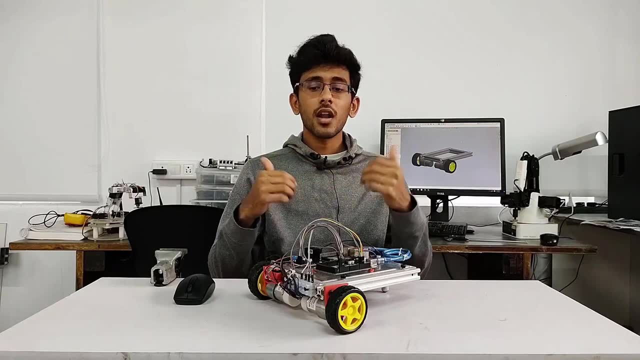 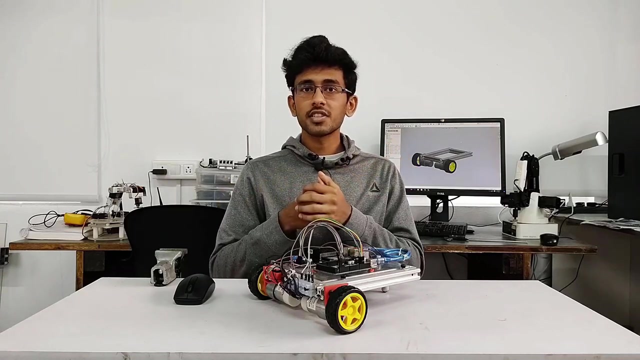 Hey guys, welcome to the channel. I'm Vinay Lanka and this is going to be a small YouTube video series on how to design and build your own autonomous rover, or AGV, from scratch using ROS. I've taken up this project as a small hobby and I've decided to document every single step. 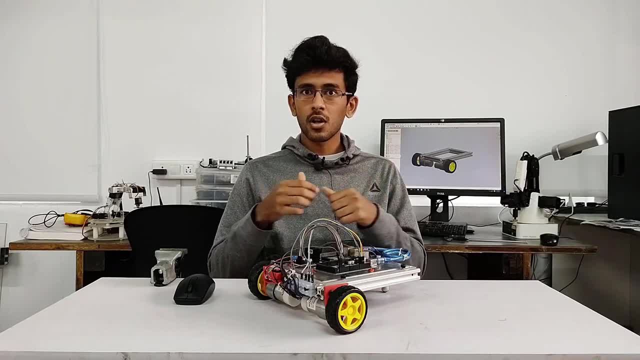 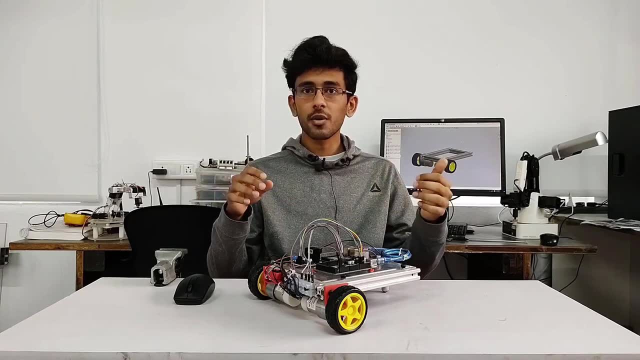 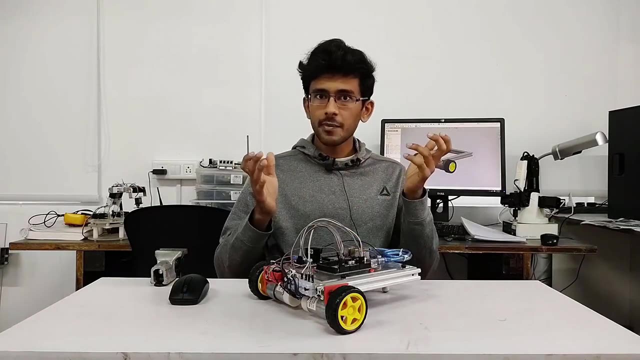 that goes into this process so that you guys can follow along and hopefully, by the end of this series, this robot is capable of navigating from point A to point B in my house autonomously, while mapping the entire area. This is going to be part one of, hopefully, a multi-part series. 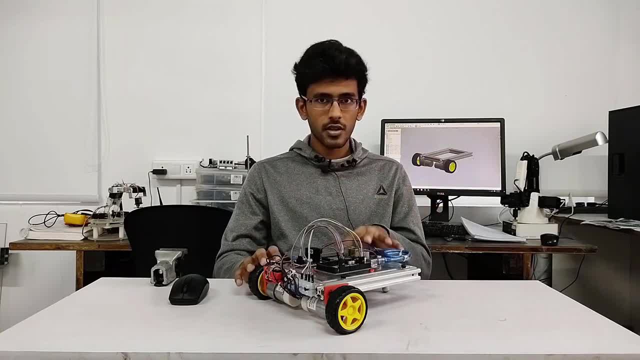 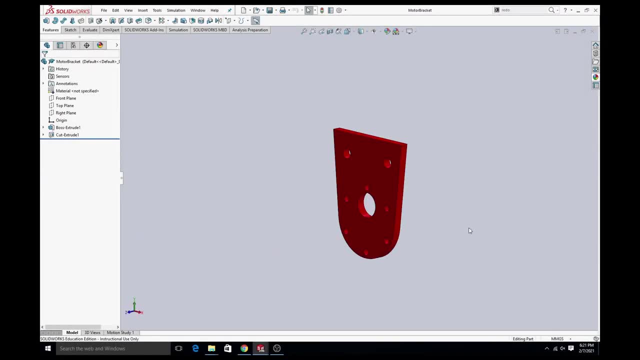 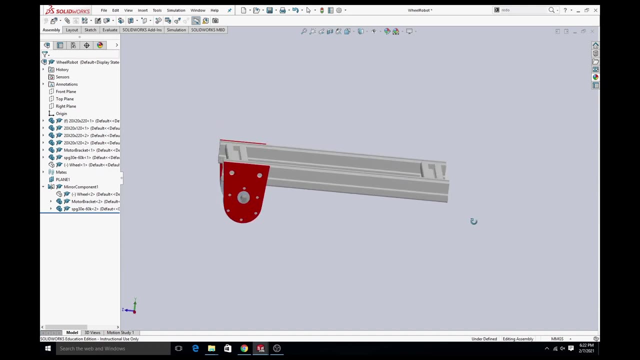 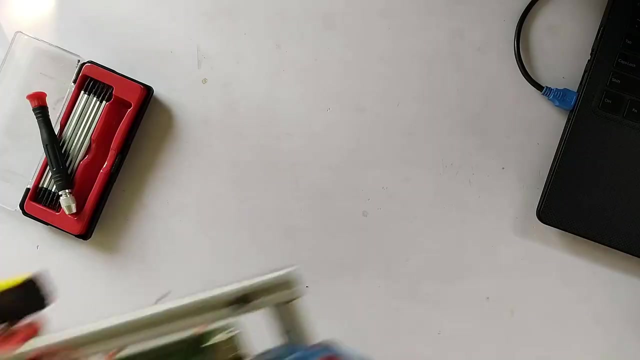 and we're going to look at how we're going to build the robot and how to get started with the Arduino. So let's get started, Okay, so let's take a look at what I've built so far Here. I have a Raspberry Pi 3, which is 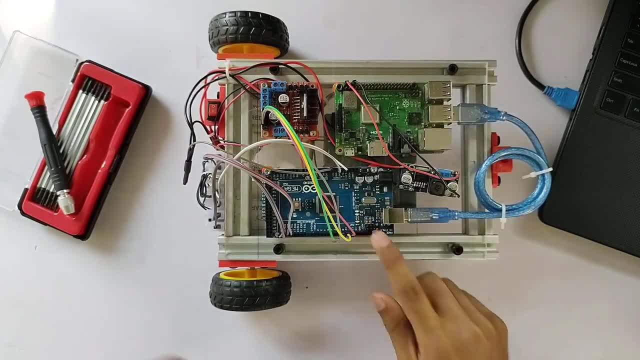 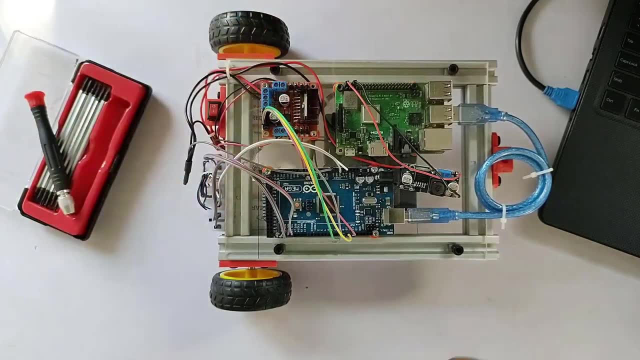 connected via a serial cable to the Arduino Mega. The Arduino Mega then drives the two motors located below via an L298 motor driver. I've chosen the L298 motor driver because I want to use it in this particular configuration, because the Raspberry Pi is suited to run ROS. We'll take 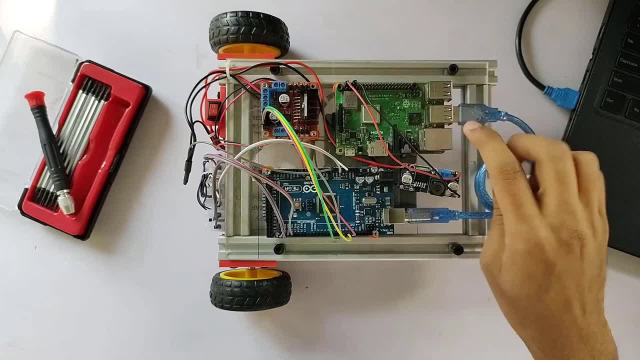 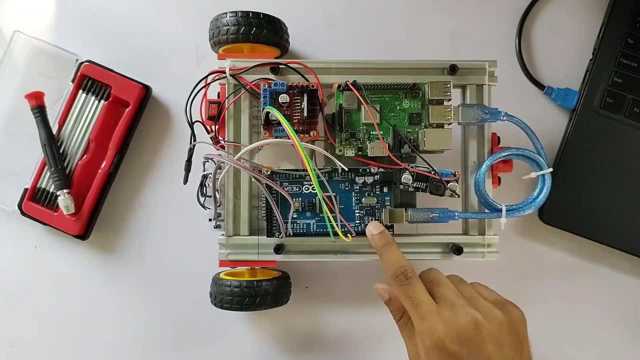 a look at what ROS is capable of at a later stage, but for now, let's think of Raspberry Pi with ROS as a higher level controller, which is issuing commands via the serial cable to the Arduino Mega, which acts as the lower level controller. This particular configuration makes sense because 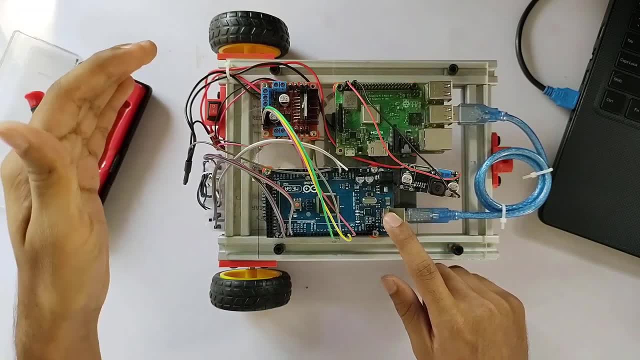 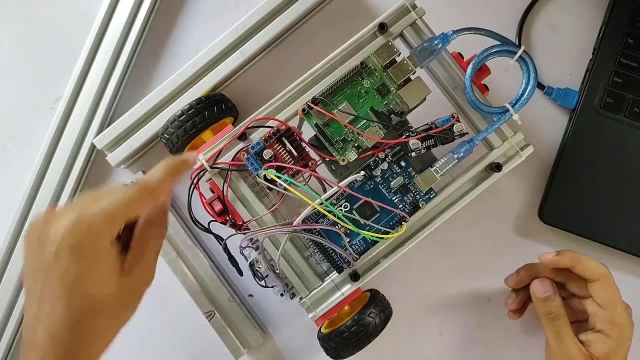 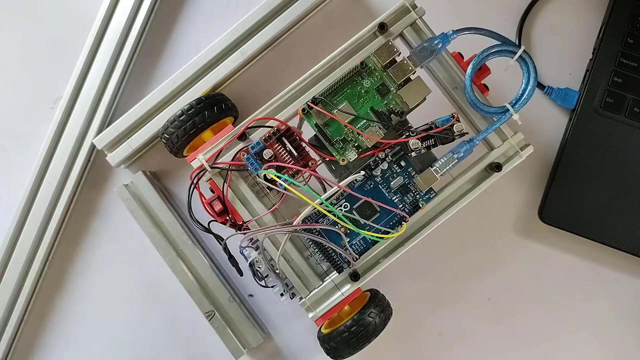 the Arduino is better suited to interact with lower level drivers such as the L293 and the motors. Looking at the design of the robot, I've based the entire design of these four aluminium T-slot channels. These channels are very versatile as they come in various shapes and can be cut to any. 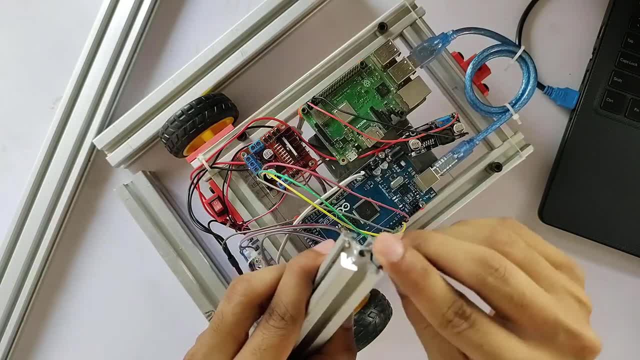 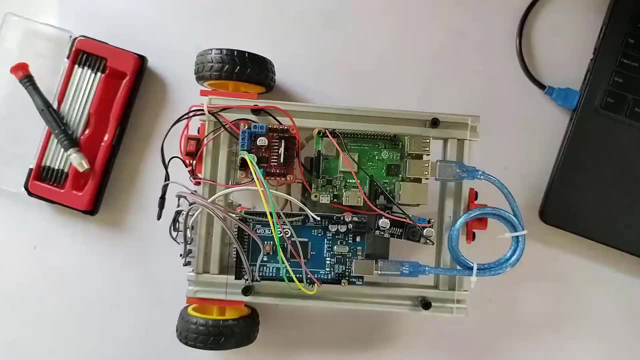 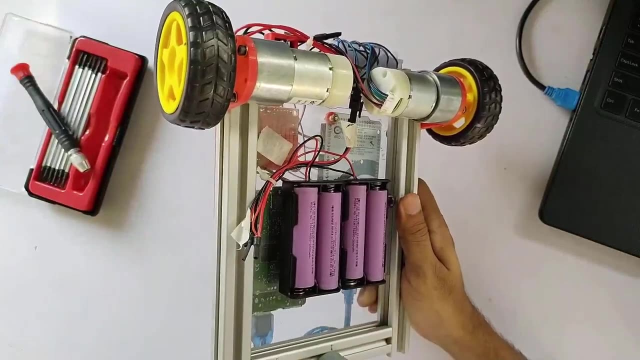 length. Also, you can fit anything from any direction using those T-slot channel nuts, which is useful when I fitted the acrylic top and the 3D printed motor bracket. Okay, so let's take a look at what's underneath. Here we find that we have four lithium-ion batteries, each rated for. 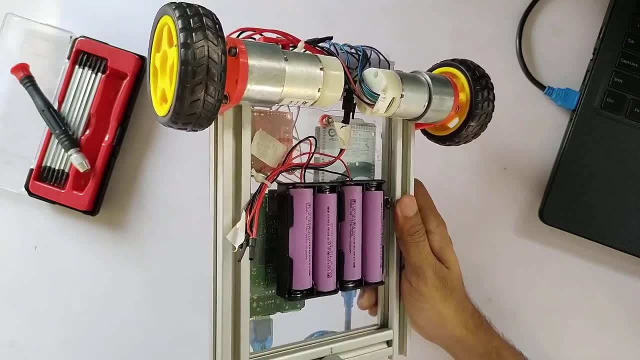 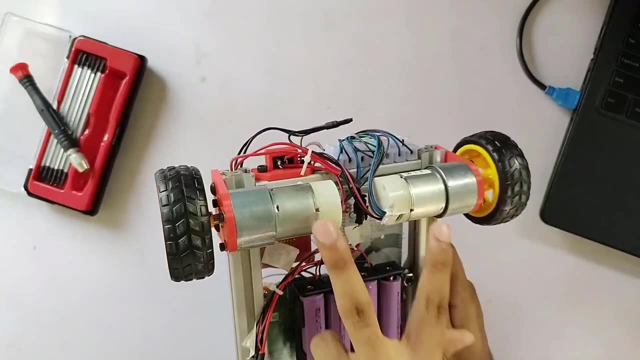 around 3.7 volts, but I find out in practice that they give around 4 volts, So four of them will give around 16 volts. Here you can see them properly. Coming to the front, we have two DC-geared motors. 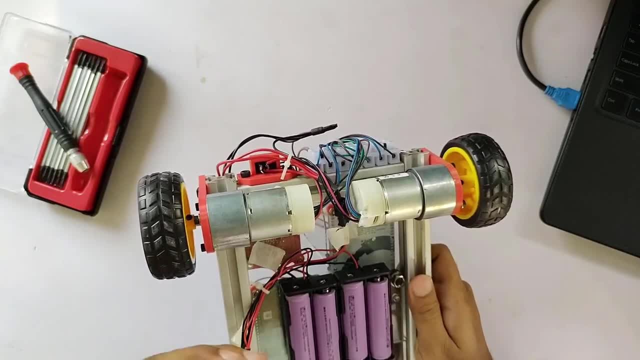 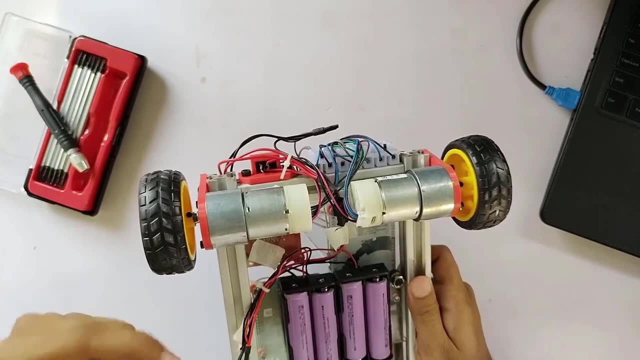 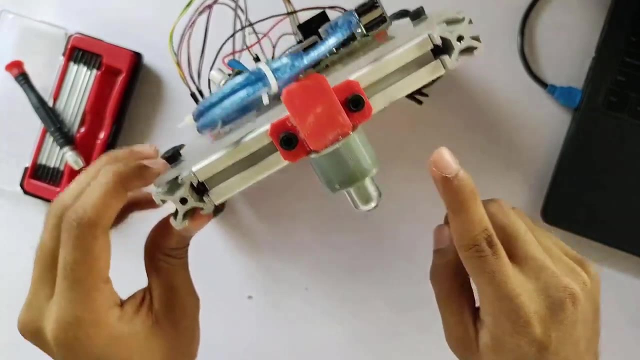 from Citron with encoders built into them. The speciality of having encoders built into the motor is that these Hall effect sensors tell you how much each wheel has turned at any given point of time. Coming to the back of the robot, here we have a casted wheel which is attached to a 3D printed 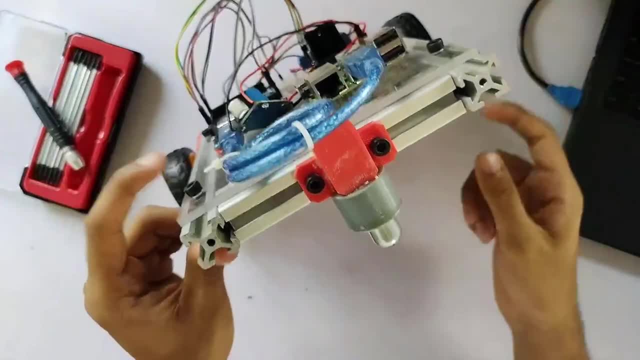 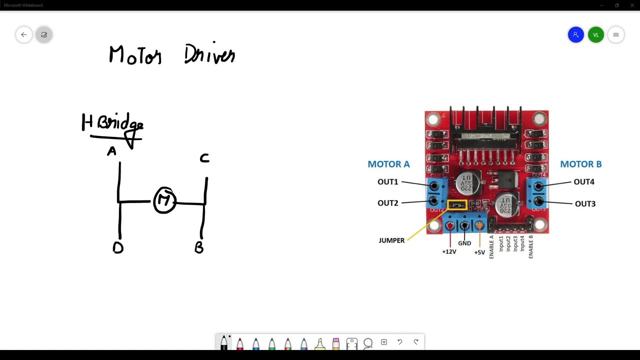 bracket. We've used a casted wheel instead of two wheels on the side, because it's easier to maneuver a robot with a casted wheel. Before we jump into writing some code to drive the motor, I thought we'd take a moment to figure out. 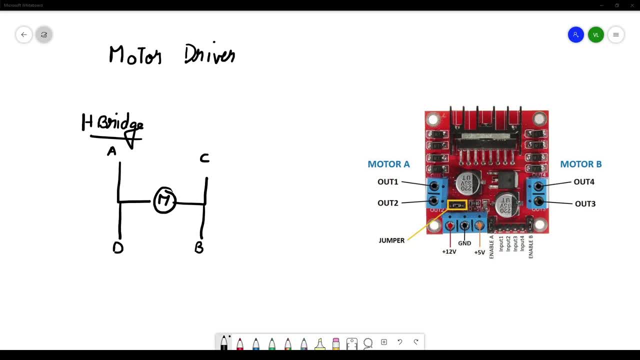 how to drive these motors. Arduino can't handle the current requirements for most motors because it operates in the milliamps region and cannot handle the current requirements of these motors, which are magnitudes higher, Which is why we need these motor drivers, The one I'm currently using. 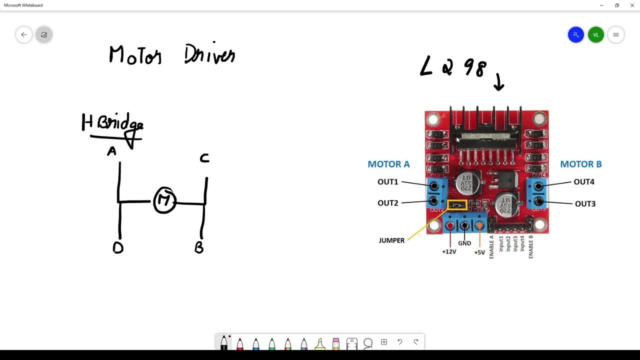 is the L298 motor driver board, which is the exact one I'm using in this project. We'll take a look at what these pins do in a while, But I'd like to highlight one important feature or concept of these motor driver boards, called the edge bridge. 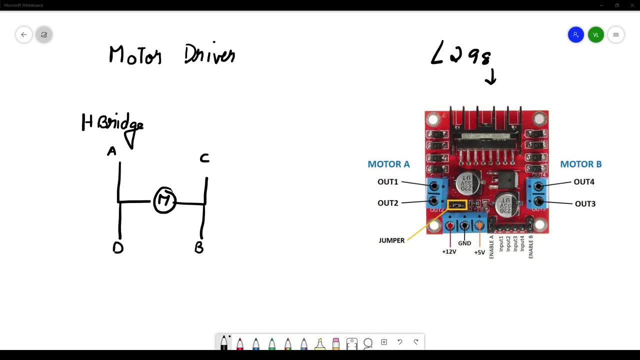 The edge bridge gives us an easy way to turn a motor in two directions. Suppose we have a motor M and to turn it clockwise we need to turn this terminal positive and this terminal negative With an edge bridge. by turning A positive and B negative, the current flows in this direction and the motor turns. 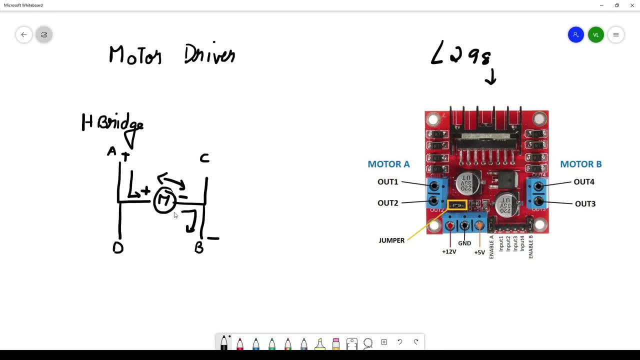 clockwise. Now suppose we were to turn it anti-clockwise. we just switch the polarities by turning C positive and D negative and the current flows in the opposite direction. This functionality is given to us by the L298 driver board, by these input pins. 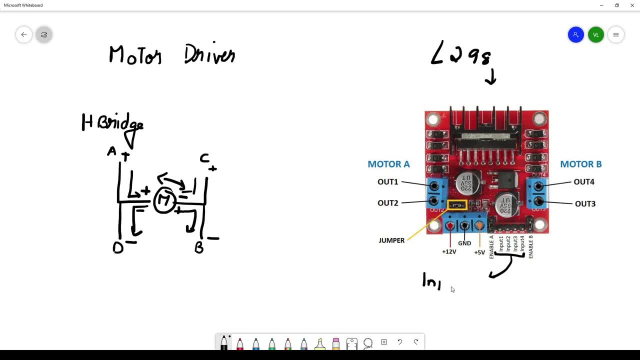 So suppose we have IN1 high. that makes A positive, B negative. turning motor A in one direction, say clockwise In turning into high will make C plus and D minus, turning motor A anti-clockwise. Similarly IN3 and IN4 will do the same thing for motor B. 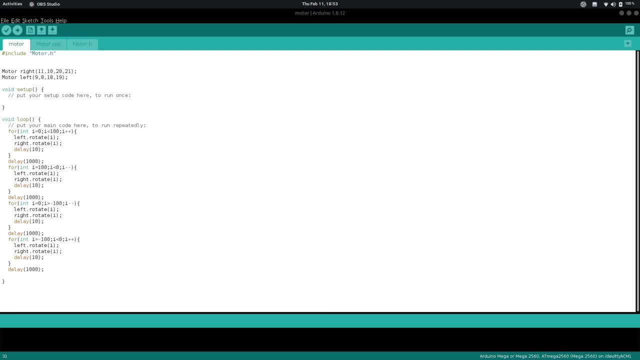 Okay, so it's finally time to write some code. This is some code to just check whether the motors are working or not by just turning them in one direction and another. Normally, at this point I just slap some input output statements in some for loops and call it a day. But this is a. 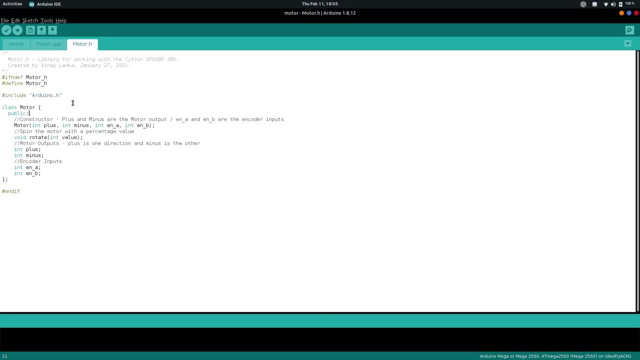 YouTube video. so I decided to step it up. I've written a class for these motors. Now the class takes in the output pins, which are the motor outputs, and the encoder input pins, And I've written a constructor to initialize all these pins. I've also written a function called 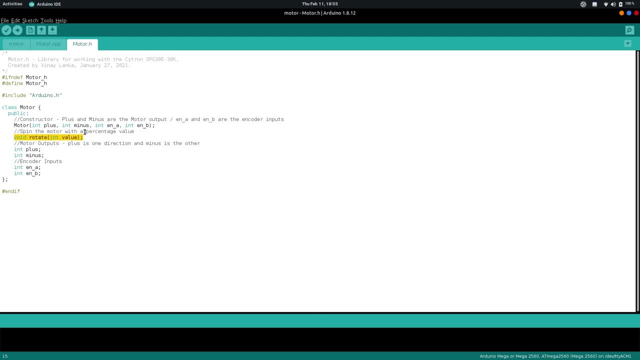 rotate. It takes in a value from 0 to 100 or 0 to minus 100, basically a percentage value, And all the functions are in the CPP file. The motor constructor function takes in all the pins and sets the pin modes. The rotate function, as I said before, takes a value from minus 100 to 100. And 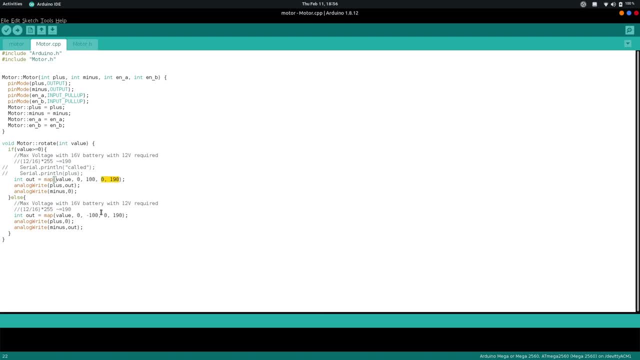 this helps them from zero to 190 if it's positive and 0 to 190 in the other direction if it's negative. Okay, now, coming back to the main program, we're just accelerating from 0 to 100, waiting for a while decelerating it, waiting for a while rotating them in the other direction. 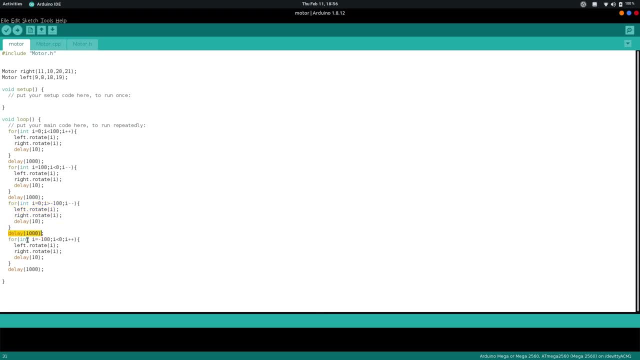 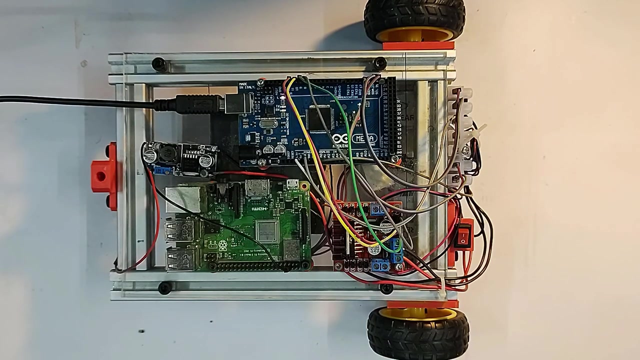 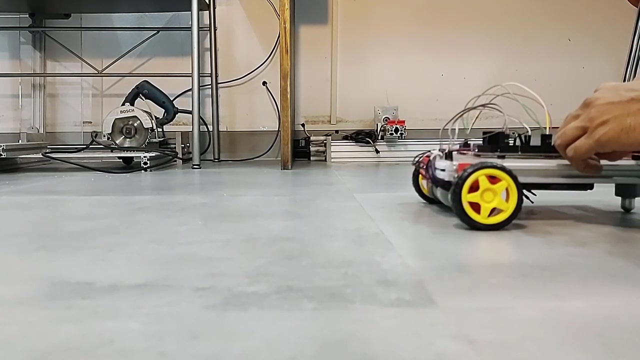 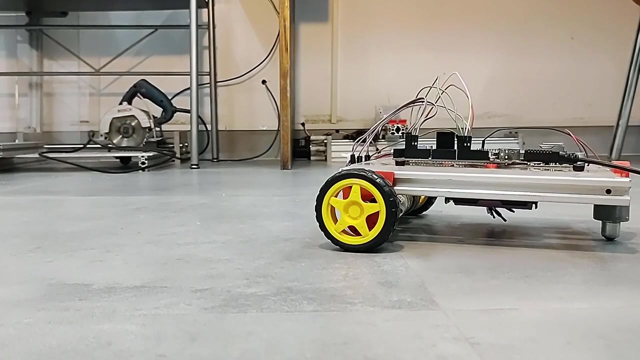 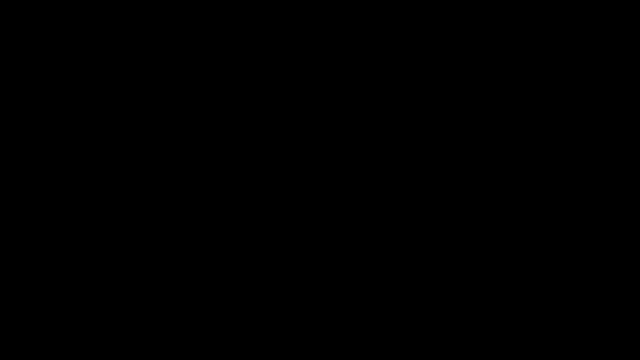 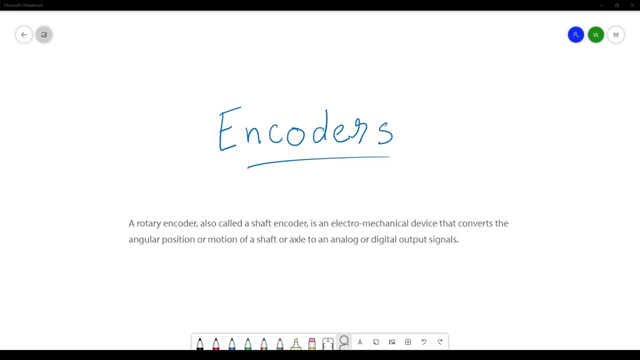 This is accelerating in the other direction again, waiting for a while and decelerating and again loops again. so let's upload it and just check whether they're working or not. time to take a look at what information we can extract from the motors using encoders. 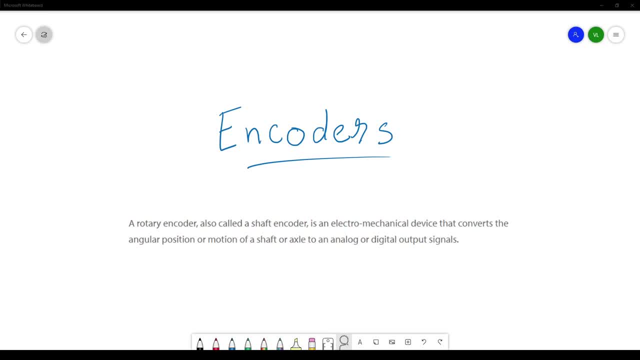 as I stated before, encoders are devices, when connected to the motor shaft, can tell us how much the shaft has rotated at any given point of time. now there are two types of encoders: incremental encoders and absolute encoders. now, absolute encoders just tell us the position of the shaft at any given point of time, but incremental encoders just 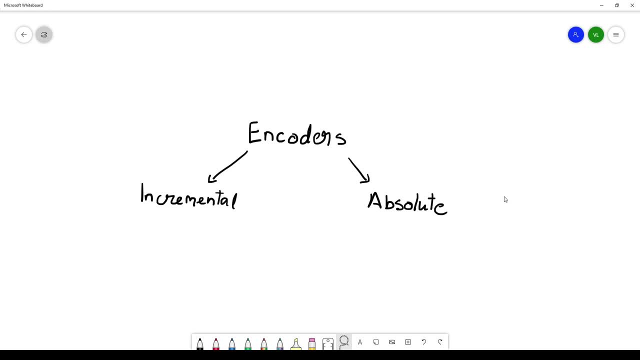 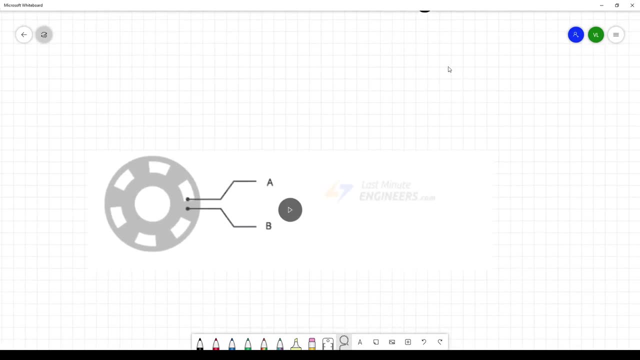 give a stream of pulses to tell us that the motor is moving. the type of encoder that I have connected to my motor is an incremental encoder. here is a gif that I found online from last-minute: engineers shout out to them. that illustrates what kind of pulses we can. 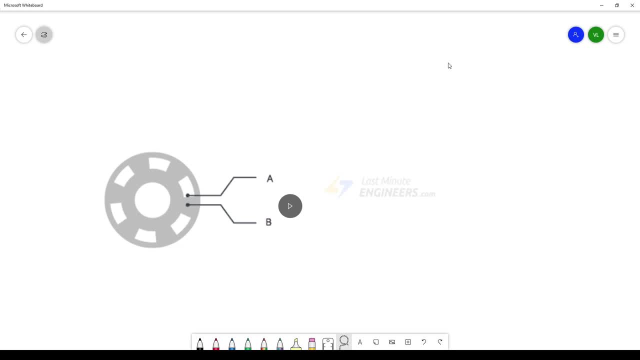 expect from an, from an incremental encoder, and how to make sense of it. so now, when you see the motor moving clockwise, you see that when A goes high, B goes low, and similarly, when it goes counterclockwise, when B goes high, A goes low and vice versa. so, using 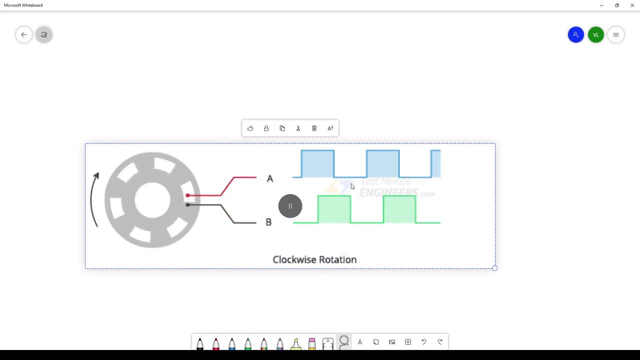 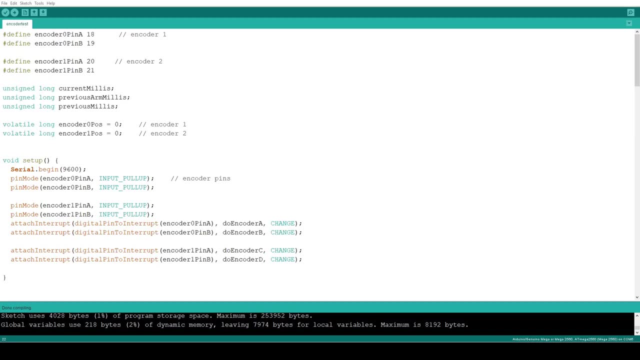 this logic we can write an Arduino program with interrupts to check what direction it's moving and how to count those pulses. so this is some code to take in the inputs from an encoder and hopefully make some sense of it. see, I'm not using my motor class, as I found out that these member functions can't be used in conjunction with the attach interrupt function. this is a limitation of the 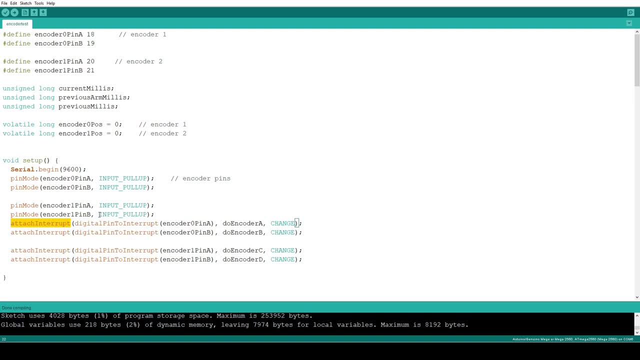 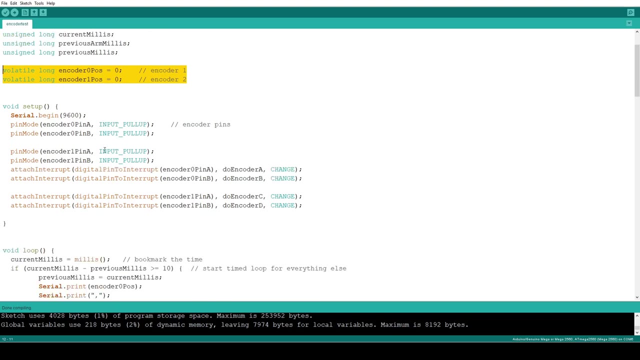 ABR language, as I found out after many frustrating google searches. but for now I'm afraid we'll just have to use the encoder pins as is, without the motor class. so I've defined the motor pins right here and I've defined two encoder position variables and 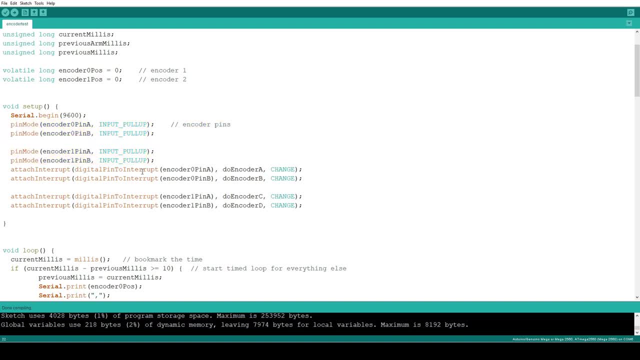 after defining their pin modes. I have used the attach interrupt function for each pin and I've given it a function to execute as soon as the interrupt has been fired. Now these functions are defined here. we'll come to that in a bit. We also have 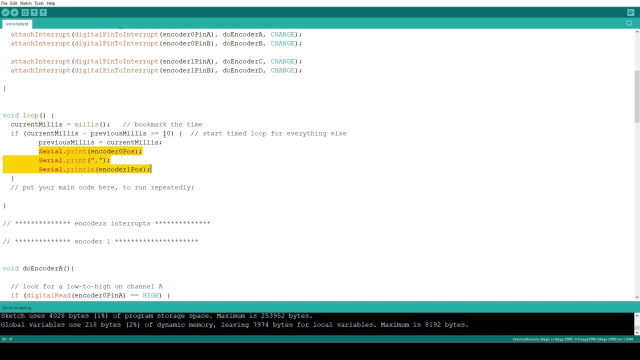 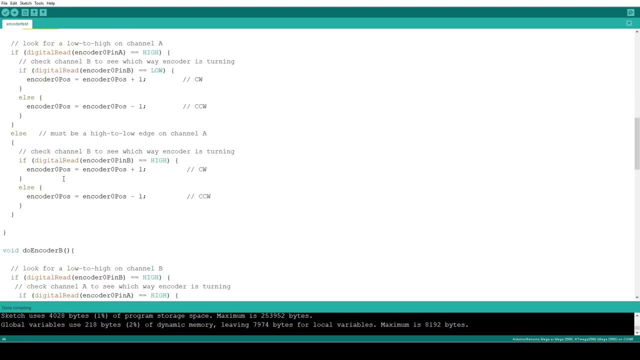 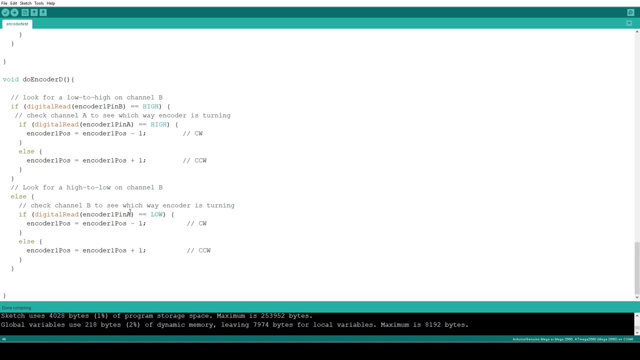 a loop that just keeps printing these positions at an interval of every 10 milliseconds. Coming to the four interrupt service routines, we've named them: encoder, doEncoderA, doEncoderB, doEncoderC and doEncoderD. I have taken these ISRs from a YouTube channel called James Burton massive.